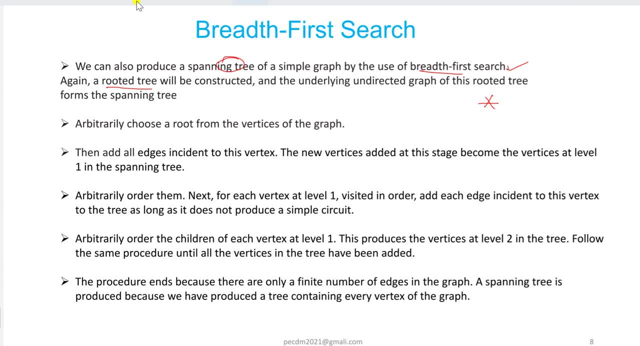 Orbitally. you can choose any element, any vertex, as a root node. Okay, There is no condition, there is no criteria. to take a specific node as a root node, Okay, ma We don't have to take a particular node as a vertex. 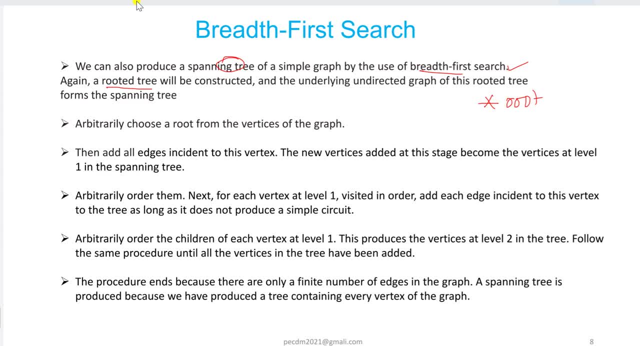 Okay, In case any elements in all the vectors, you can choose any one as a root node. In case any elements in all the vectors, you can choose any one as a root node. Okay, In examination, if they ask particular node you take as a vertex, particular vertex you take as a root, then you can choose that particular vertex as a root node. 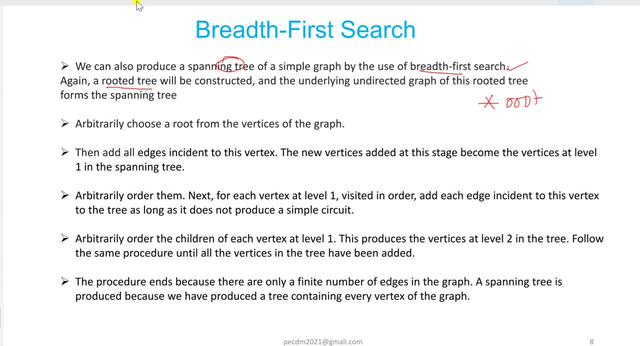 Otherwise, you can choose any one of your choice. Okay, This is the best thing in this BFS and DFS. Next Second one: what we have to do now. you are in the root node right Now. explore this particular vertex. 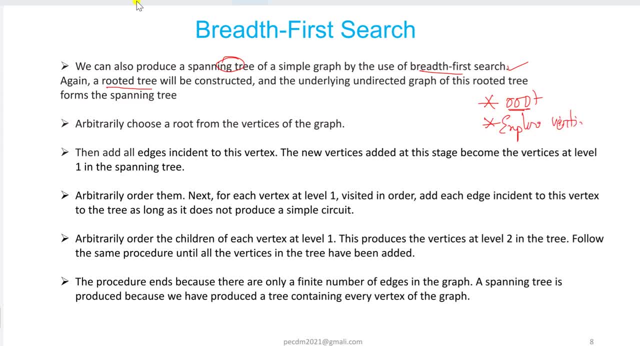 How we can explore this particular vertex into All the incident edges with this particular vertex. Okay, In DFS, what you will do: You choose the root node and second step. only you have to choose only one vertex which is incident with root node, irrespective of other one. 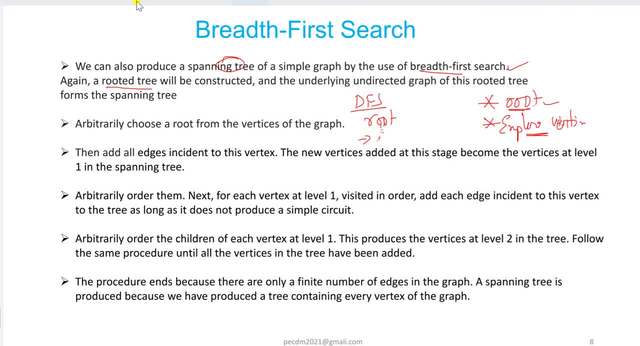